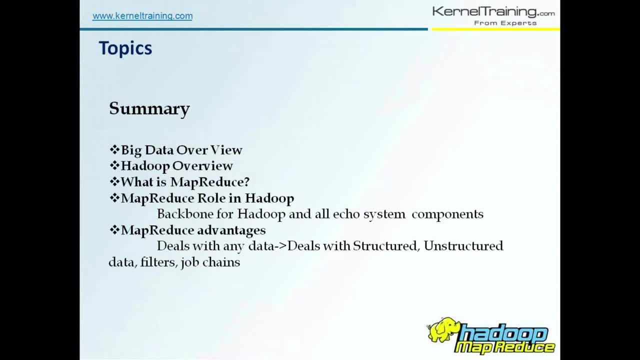 and how you get the job opportunities, what you need in MapReduce kind of thing, a brief description When we just take the training session. that time I'll give full details about what MapReduce or which work. what are all the Java classes? 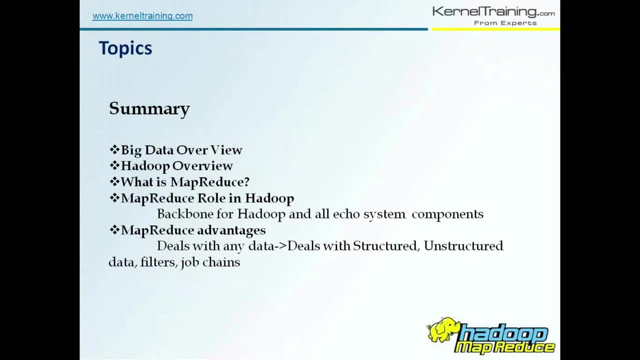 and how you need to write programs, how you need to learn all the things. I'll give you the description. See now MapReduce role in Hadoop. what is the MapReduce role in Hadoop? Hadoop has some ecosystem components. 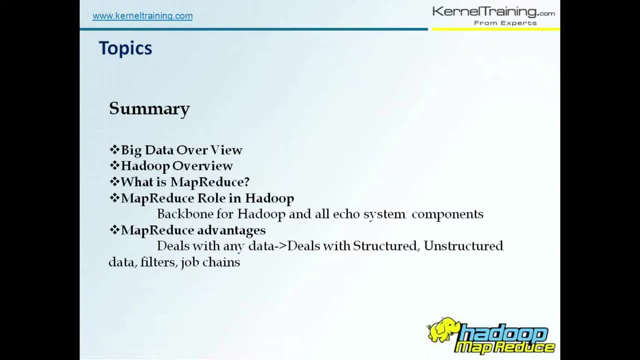 so what is its role in that ecosystem? components That we'll discuss And advantages of MapReduce. what it will do, see, it deals with the structured, unstructured data and it filters also what it filters. actually, it filters the files and the job training. 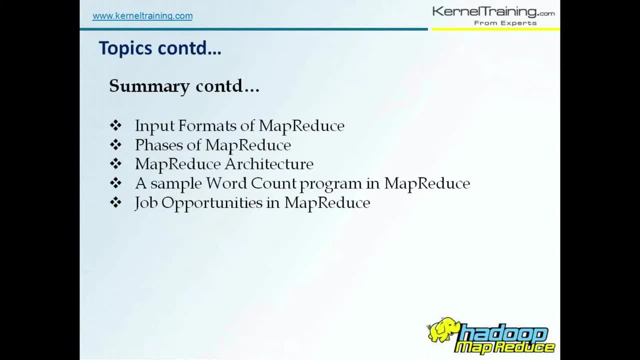 all these things we'll discuss, And the next one is summary continue. What are the different input formats it supports? Because now in RDBMS you have a defined structure data, So here in Hadoop it is not that. 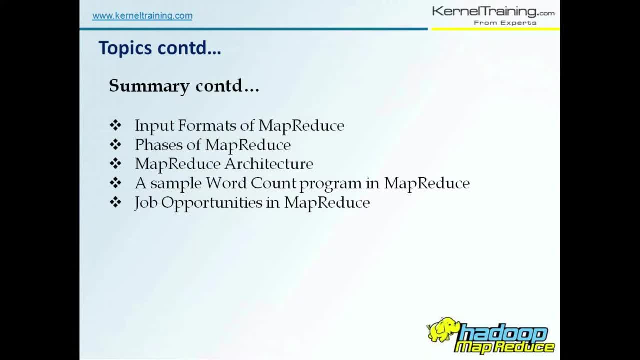 It can deal any kind of the data, So it has to support different input formats. So what are the formats it supports MapReduce that we'll discuss, And what are the different phases available in MapReduce? Next one is: what is the MapReduce architecture? 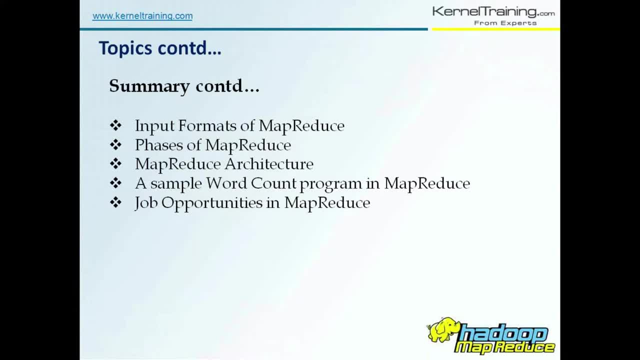 There's a simple architecture. I'm going to show you How it will work. what are the different phases in that one? Given the training details I'll give you, And the simple word count program in MapReduce- A small program usually. 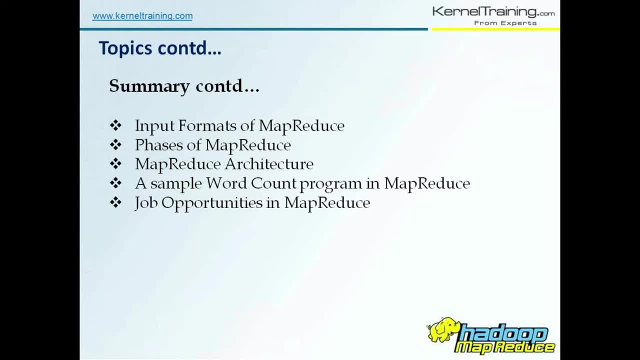 It's like counting the words I have taken. So when this passes through different stages, what happens And finally output is generated. How output is generated I'll show Last. the job opportunities are available in MapReduce. Hadoop itself has a lot of potentiality scores. 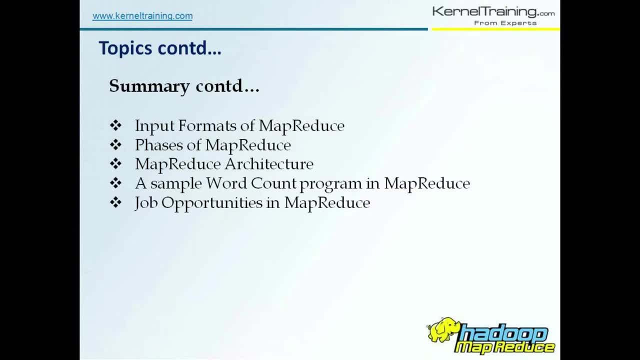 Within that scope, what is the role of how you get the MapReduce jobs? I'll show you later. If you master the MapReduce, that's all. They won't see any other ecosystem. If you say that I have no good in MapReduce, I'm good in Java, that's all you'll definitely. 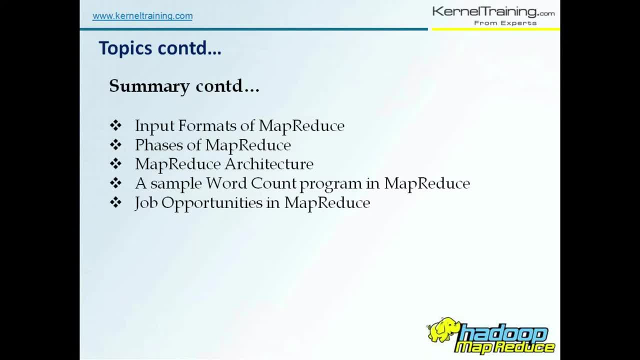 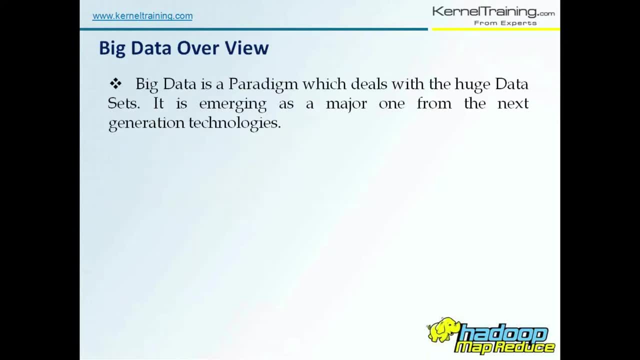 get the job in Hadoop. If you do not know the other ecosystem components also, they don't care. They need MapReduce because it's the core, basic component of the Hadoop. demo of the MapReduce, See. now I'm going to give the details. 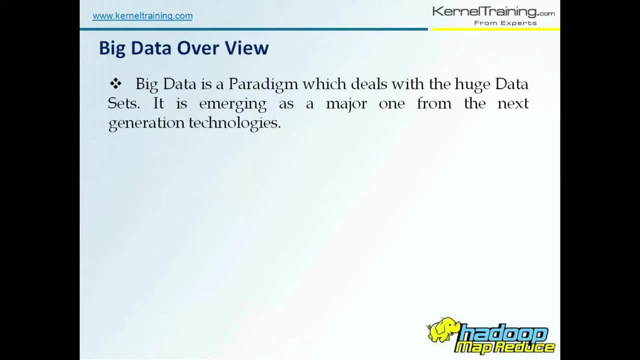 What is big data? Let us see a small. big data is a paradigm that deals with the huge data sets like huge data sets. It's like a pet up. Also, it's not saying that I'm just good in Java because it knows Java, that's all. 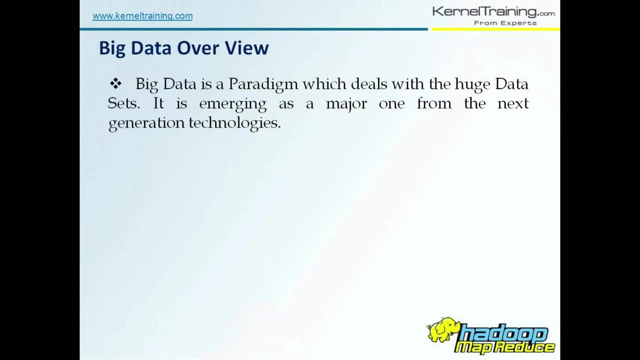 With these three types of technology it does not go to the job because everybody, almost all persons, know heavy competition in that area. You should be an extra knowledge you should have, and the emerging technology knowledge you should have, then only you can sell yourself, you can get the job. 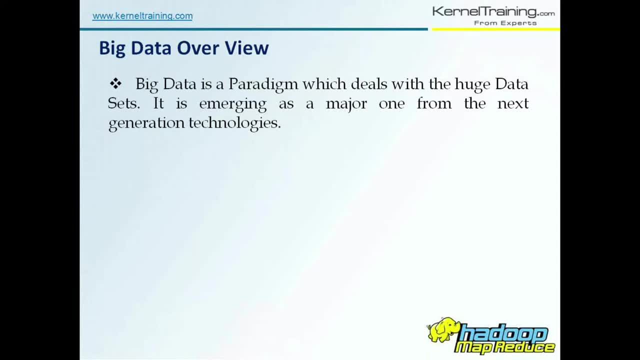 That's what this big data. it's a very powerful emerging technology in the analytics field. it comes Because now, cloud computing, mobile technologies, analytics- these things are emerging technologies- Out of this analytics category, this big data comes into picture. 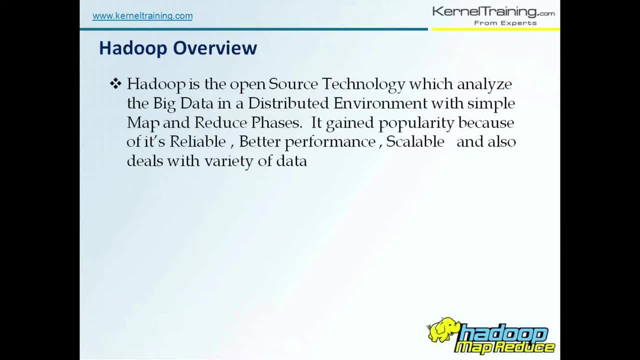 So this is: what about big data? Next, the Hadoop value. What is Hadoop? Since big data is the one paradigm, Hadoop is a tool which implements the big data. That means it's an Apache, open source tool which works on the big data. 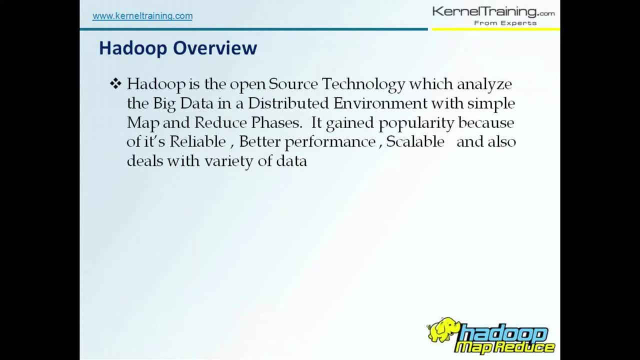 It's a huge data sets How it is doing that one. it puts the data in a distributed environment, in the sense that data will be divided into separate blocks and put into different nodes, and then each node will process the data separately and finally all the data is aggregated and finally, 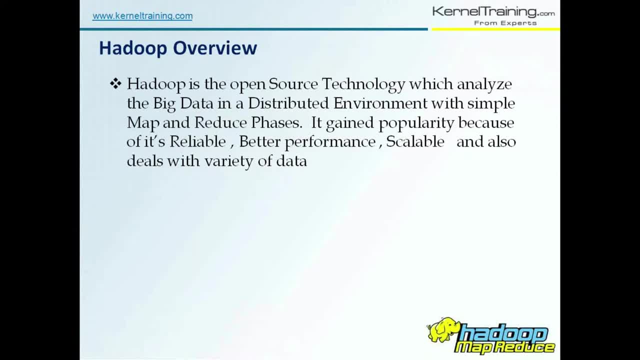 the output is generated That way because I already told that if you want to load one MD file it will take five minutes. Suppose 10 MB means 10 minutes. like 200, GB means two hours, four hours, like that it will. 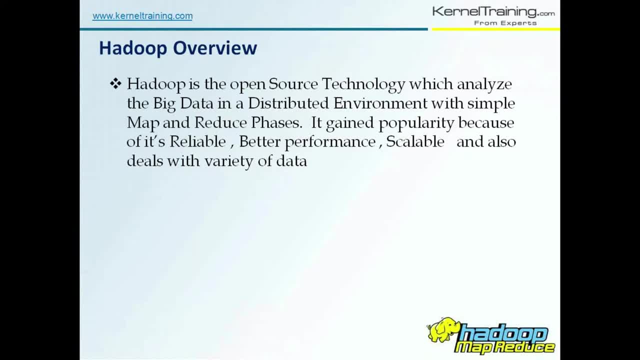 take loading a cell phone. So how can you just work on that data when it's a huge data set? So you can't work with a single system. that's what Hadoop comes into the picture. It distributes the data, divides the data into blocks, put into the cluster and then 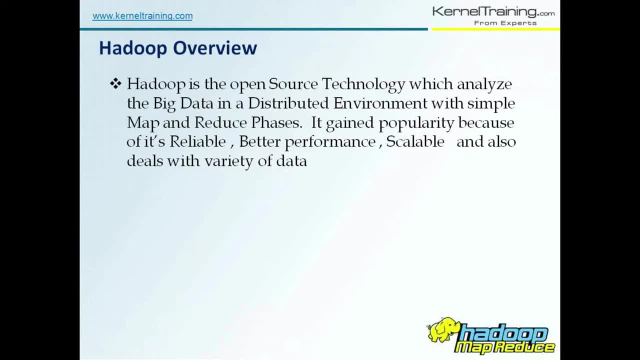 process it. Finally, output is generated. That's what. So within that it has two phases, like map phase and reduce phase. Why it gained the popularity? Because of its reliability, because how it is reliable means data not only, it is splitting. 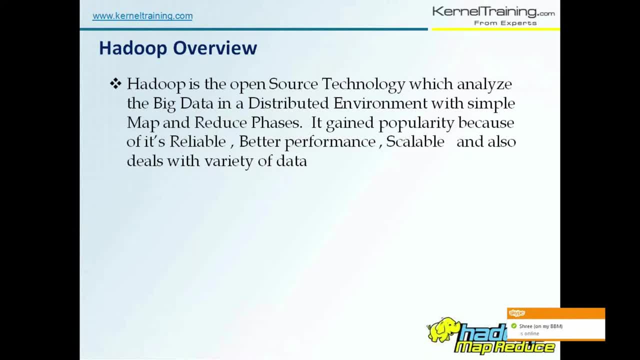 the data. it also duplicates the data into different nodes. That means, suppose one node is failed, it automatically picks the data from the other nodes, start processing. That's what it is reliable And the better performance. Suppose you have 10 nodes. 10 machines are there, the data is loaded into 10 machines. 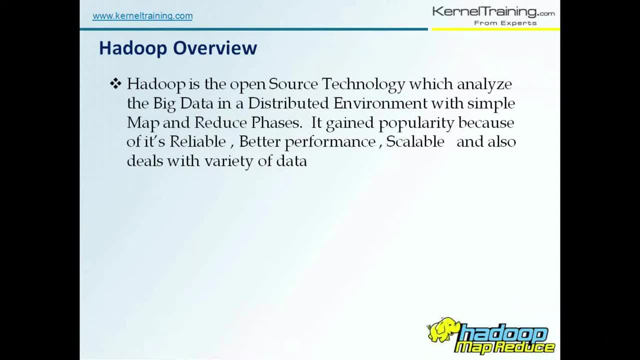 One machine started not working. So what will happen? Immediately, the framework will look into that one and see this node is not working. Immediately it asks the other node, yes, available. It acts the same job to execute from the other nodes, That's all. 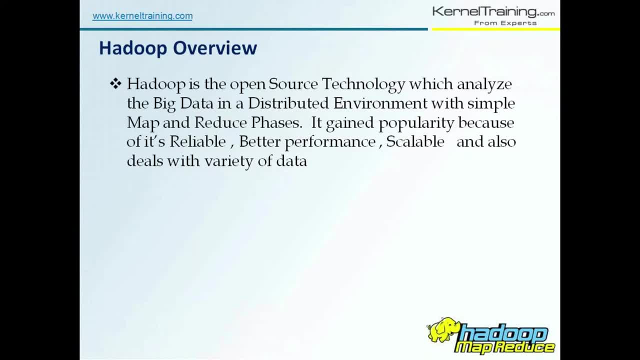 When this node gets ready, then again it will just give the data, Again, it will just give the work to this node. That way the performance is achieved And another one is scalable. What is scalable? actually Suppose the ability of software to perform when suddenly a number of VCs increases. 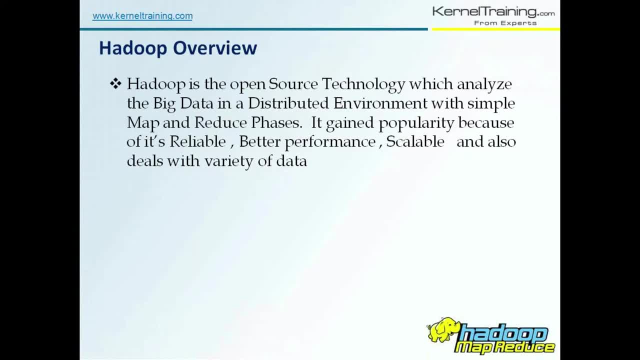 Like suppose there are 10 nodes, Suddenly, if you increase five nodes, how it will perform, How it is do what it will do, that kind of thing, So that here it is scalable. That means there are 10 nodes working. 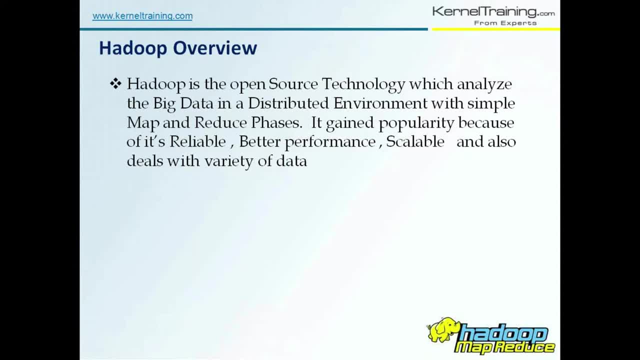 You want to add two nodes in the production environment Without any much disturbance of the job, you can easily add the nodes. Similarly, you can degrade any nodes, remove any nodes from the cluster. You can add the nodes from the cluster. That kind of the flexibility is there. 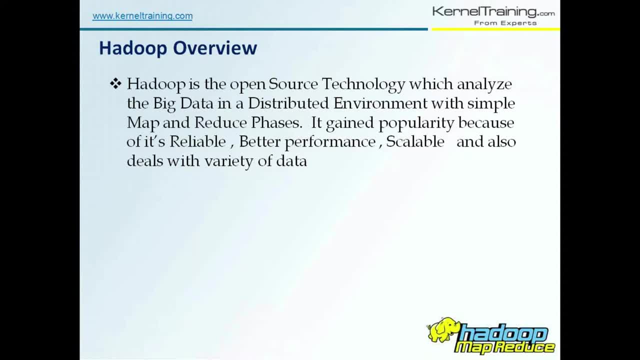 That's what Haroop gained the popularity: because of the reliability, performance, scalability. It deals with the different kinds of the data formats, But yet simple technology like map and reduce two phases- only These two phases- deals with the data. That's what. 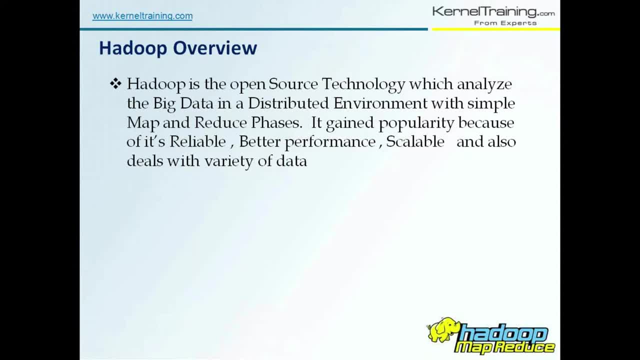 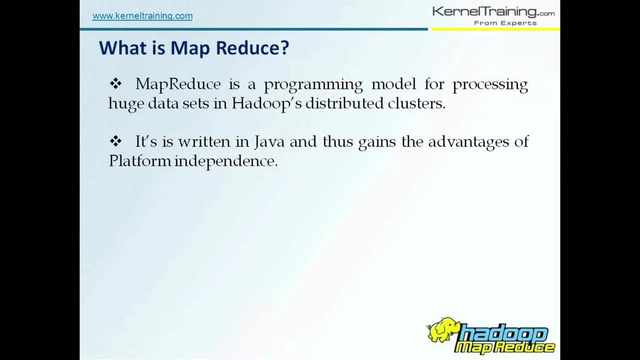 You just appreciate this, This one, when you just go through all the sites and finally, you just appreciate how this MapReduce is doing this job. What is MapReduce? We know about that big data. We know about Haroop. What is MapReduce here? 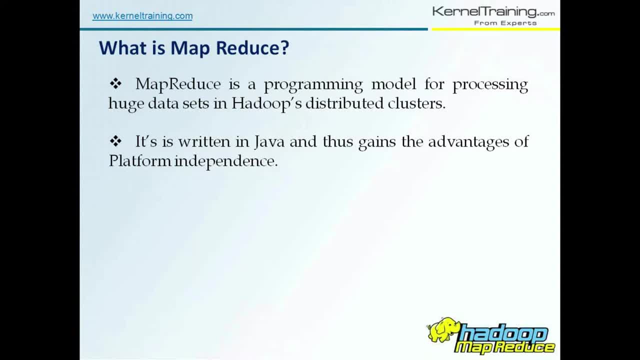 MapReduce is a programming model which deals with the huge data sets in Haroop distributed clusters. MapReduce is the process one because it's a core. It has to process the data Haroop. Haroop uses the MapReduce to process the data. 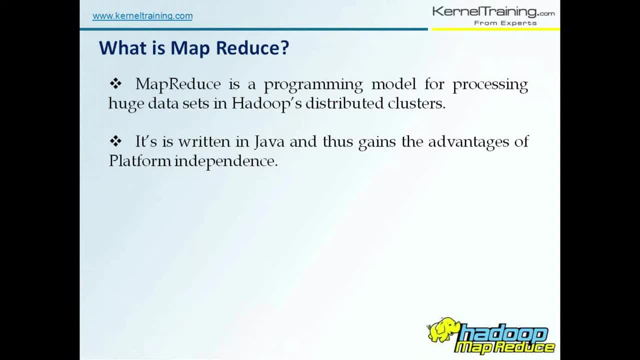 So it is written in Java and thus it gains advantage of the platform independence, because since Java is write once and run anywhere concept, So if you write it in a Windows here, the Java program, the same can be run on the machine, Macintosh machine, and also like you can run it there in the unique systems also. 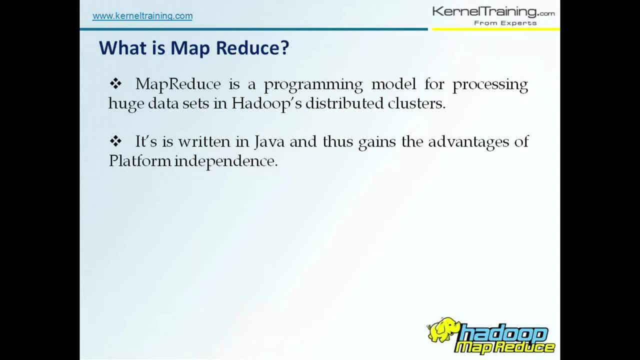 It has advantages. And also one more thing I can tell: the streaming facility is also there in Haroop. that means, since, though it is developed in Java, It fascinates the other programming languages like Python and other languages can pick up this data, because streaming facilities like the output, the data is generated to the output. 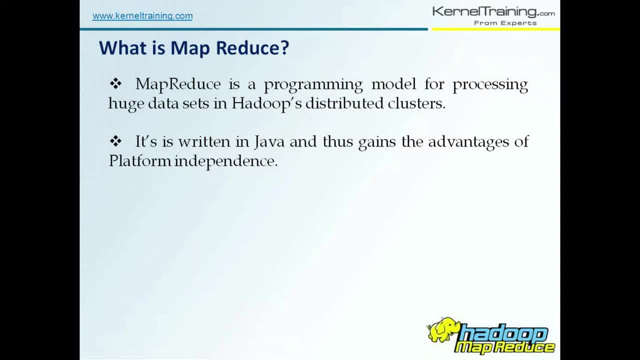 and from output the other languages pick up, picks up the code and then finally it gives the. it works on that. So this is what: streaming. This is also one of the major advantages of Haroop. Next one: Role of MapReduce in Haroop. 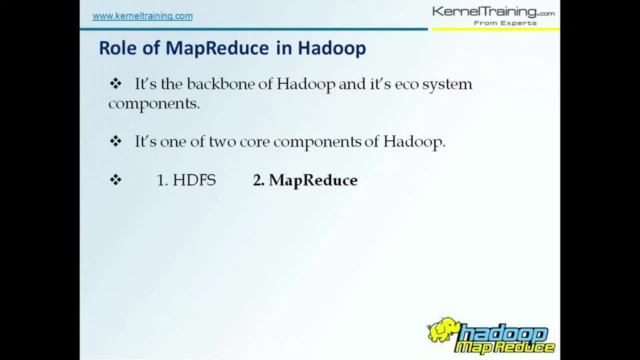 Like it's a backbone of the Haroop and it's ecosystem components- Most of the Haroop ecosystem components- back end it will run on MapReduce only. For example, PIG is there. PIG is a scripting language but back end MapReduce only will run. 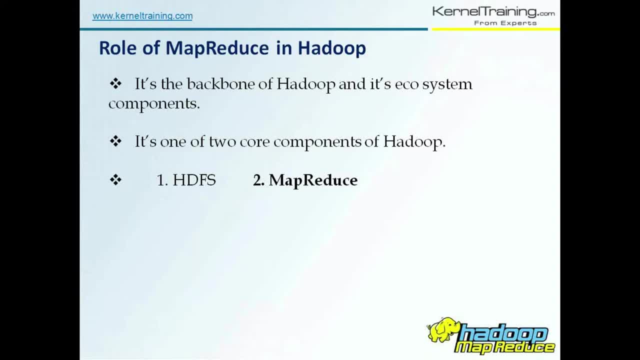 Java program will run, Though if you can see that we converted it to MapReduce jobs and similarly, Hive is the database language. If you write the query, the query is automatically converted into the MapReduce jobs and finally, in the back end it runs the MapReduce jobs and produces 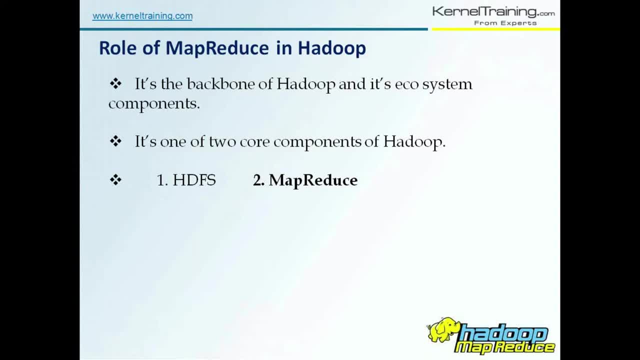 Like how you, if you know about Java JSP, the JSP is converted into the sublets and finally in the back end servers will be running Similar way. it is like any PIG and other Hive for back end. this MapReduce only will be running. 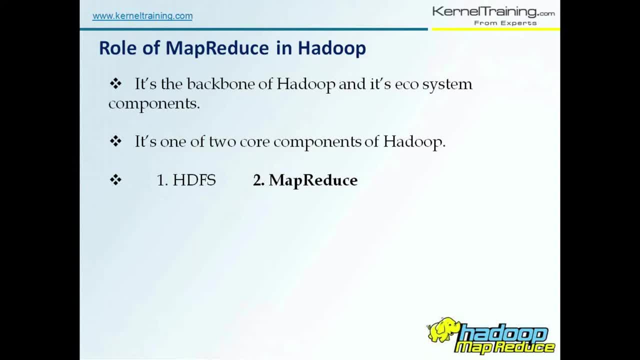 there. It is one of the two core components of Haroop, like see when I say that it is a cluster. there must be another technology to read and write the data because if it is a single file, you can read and use the other, use the existing file system to read the data. 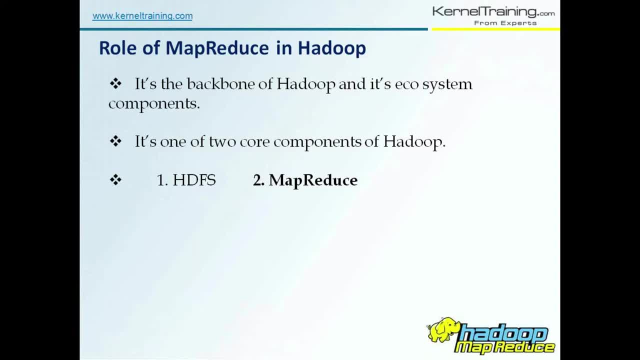 But whereas this is different, data is physically split into blocks and put into different nodes. You should have a special technology to read that. That is what HDFS- Hadoop- Distributed File System. That means: if you want to put the data you have to Hadoop, HDFS will just split the data. 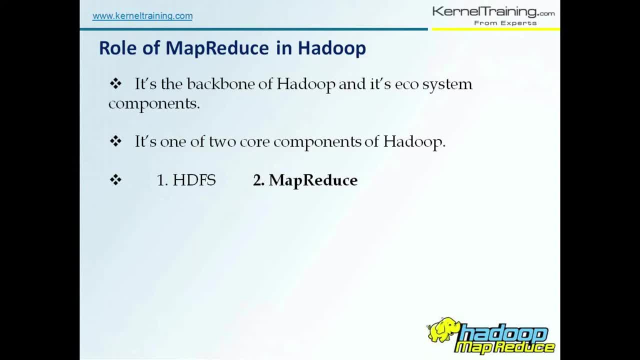 and put into the cluster. and, similarly, if you want to read, it will read from the cluster. That is what HDFS- HDFS is for file system and MapReduce is for process. Yes, you have that file system with you. then how you process the data, how you read the 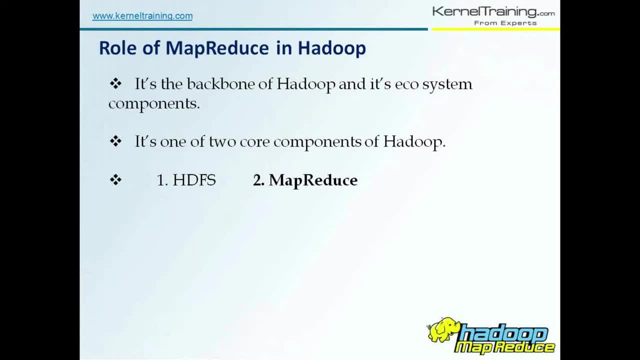 data, how you just write the data into the cluster. this is what the MapReduce and how the data has to be: different data formatting, how it has to do, how it has to read the different formats, different data- all these things related to here, MapReduce. 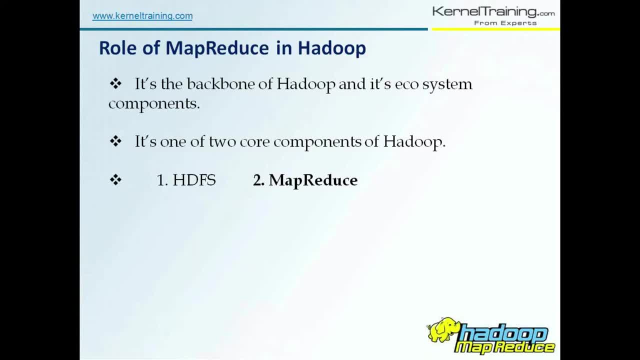 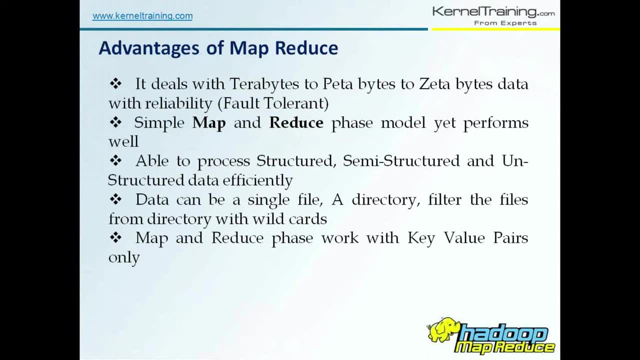 So it is one of the major core components of the Hadoop. without MapReduce there is no Hadoop. you can say Advantage of the MapReduce like see how it is: It deals with terabytes to petabytes, to zettabytes, to any huge data, with the reliable, reliable. 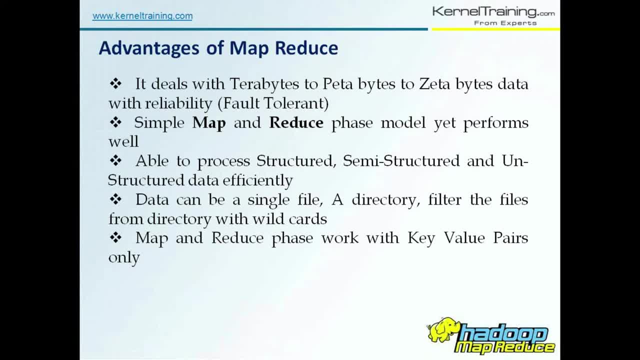 default data. So I said no earlier that when there is a node failure, immediately another node is given the job. And another thing is- though it is a huge data- very simple to phases, like a map phase and reduce phase model. This Hadoop works in two models: MapReduce will work in map phase and reduce phase. but 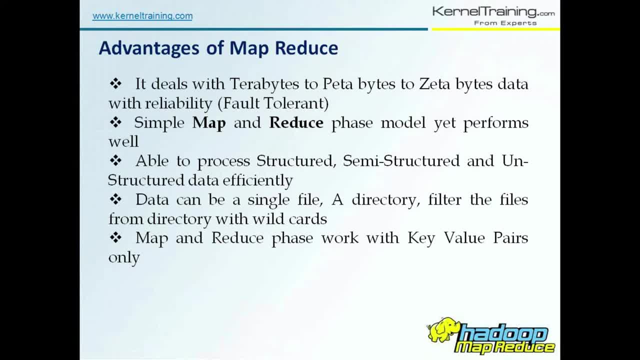 it performs very well. That is what. There is no complexity here, like a complex programming will be working, not like that. These two phases will only deals with any kind of the data So flexible, like Ability to process structured. structured data is having a definite schema, like RDBMS. 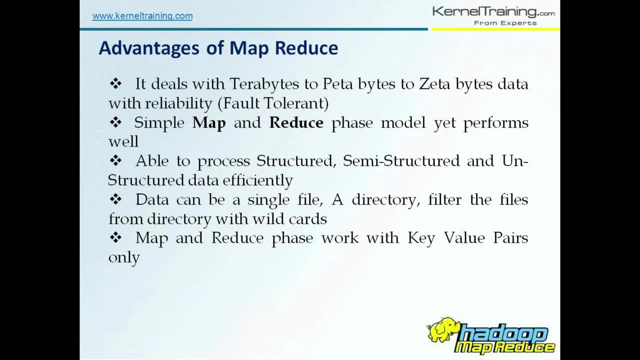 data with column, like row column kind of thing, and semi structured data like XML files, like it is semi structured data. It is not like it will be in a, It is not like it is in a. And also unstructured data like emails, text data or any video files or any of the data. 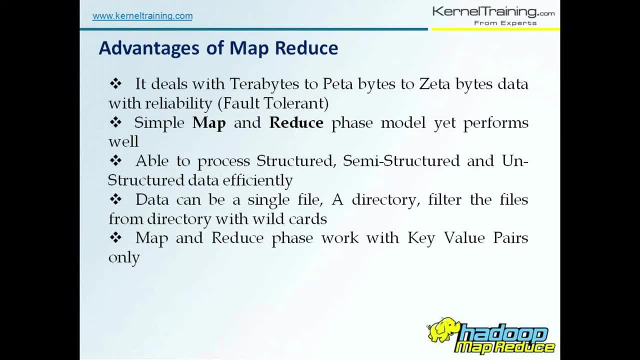 it will handle that. So that is what it has: the flexibility of failing any kind of data, and data can be a single file. That is what A single file, you can put the data to the MapReduce job. or a directory- directory containing file and files, you can directly, immediately, give the directory for the job process. 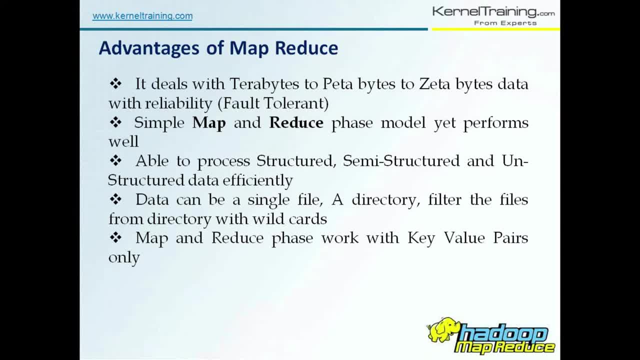 And also files from the directory with wildcard. that means filters the data. Suppose I have five hundred files. Suppose I have five hundred files In a directory. I need to select the files starting with A or I need to select the files starting with D only. 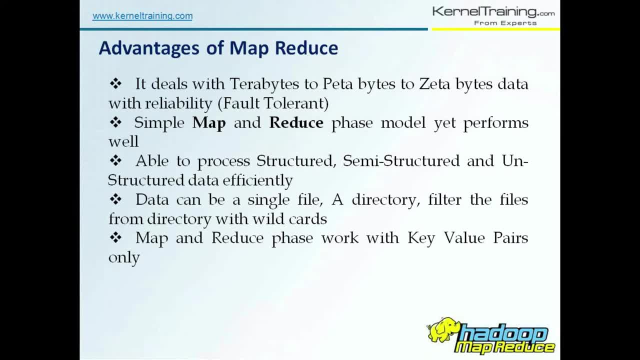 You can specify in the job that starting all the select all the files with D, star, dot or you can extension also you can filter it, that kind of thing. So out of the five hundred files, whatever that filter, you are giving that kind of the files only. it picks up, then runs the MapReduce job. 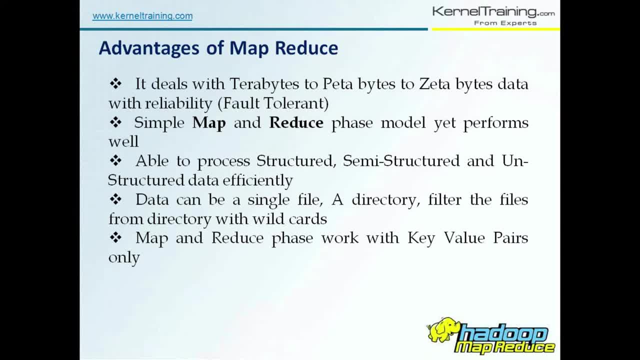 See how flexible is the advantages of this MapReduce. It is a. It works on the different, It works on the different data types and the other side is like different files can be handled by filtering and a map and reduce phase work with key value. 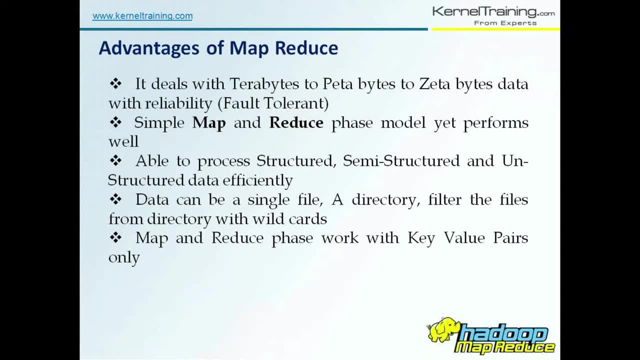 Another thing is like a very basic thing. very important thing is it works with the key value based on, not like any map. also reduce with both of them will work with the key value based on. Key means key comma, value based, Right, That kind of thing. that only it was, because whatever the data is given to MapReduce, job. 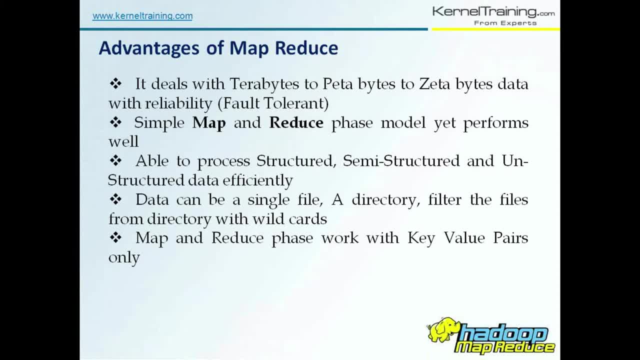 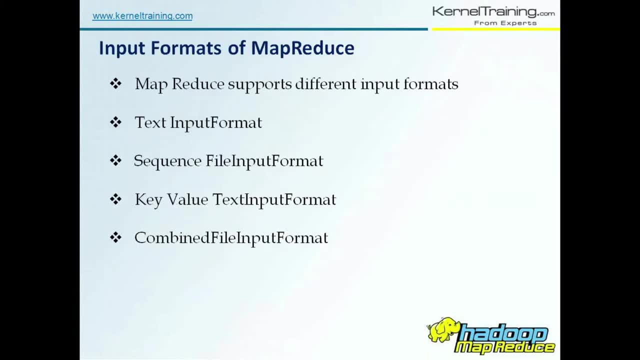 it automatically converts that into key value and started processing that. if you have one key value, What are the other things with that key? when you can extract it that way, you know we can accept. you see that one in the work on problem: how it and what are the input formats that. 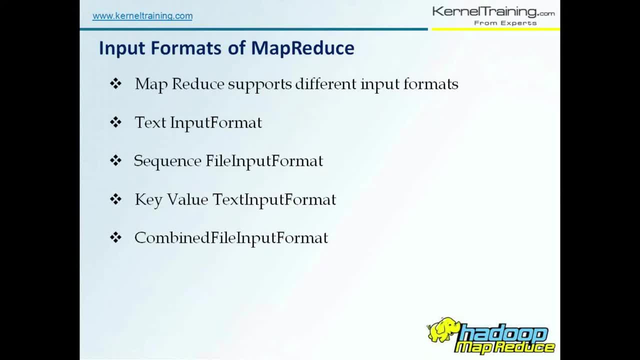 MapReduce- Because I said no already, there may be different kinds of the data- is fed into the MapReduce job. How it will work: See it has this support formats: Test input format. If it is set, it will process that using that input format and similarly sequence file input. 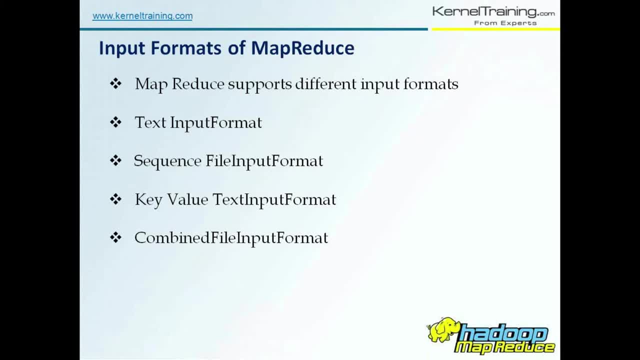 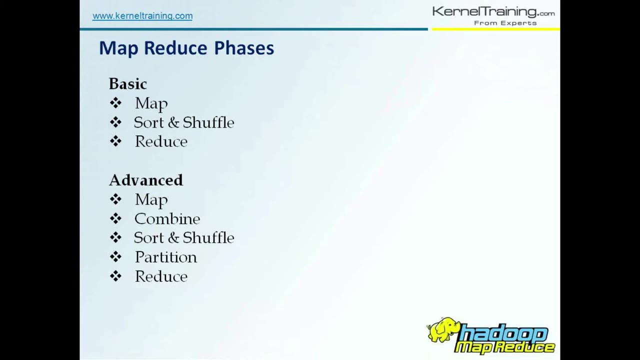 format. If it's a sequence file, it can. is that even for zip files? and now it is with the markets, some combined file input format? And also we will discuss that the details about in training or different input formats and how it will handle the MapReduce phases. 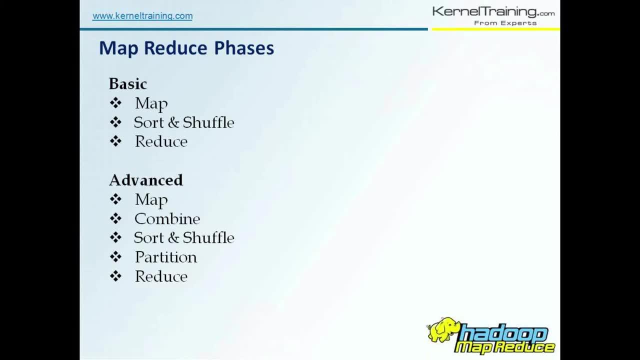 What are the different phases available in MapReduce? Basically there are basically. there are three phases like map phase, soft and shuffle phase and reduce phase. It has to map the data first. That means I was telling in the previous demo, also in Hadoop, out of the hundred percent. 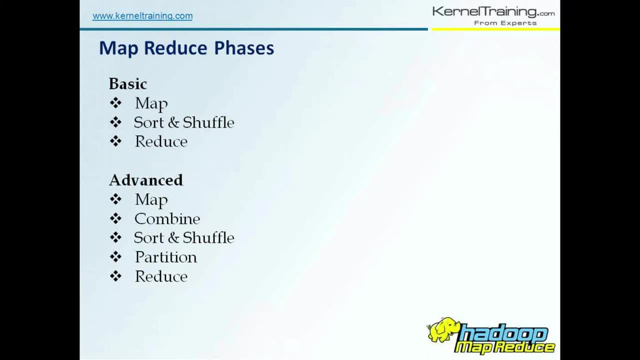 of the data you may require only twenty percent of the data only. that's all Other data is not required. So what it will do? it map the data only. suppose there is one weather data, for example. it doesn't have any specific fields. like it is running data, it is within that data you need to pick. 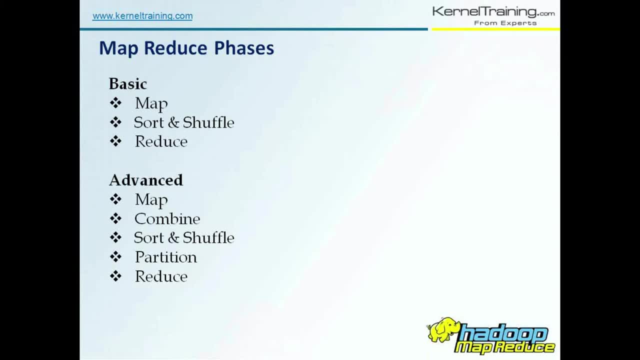 up. the fifth character to tenth character is data. So that's all. The fifth character is a temperature, suppose, as you. So it will go and pick that fifth character, only the rest of the data it leave it. it doesn't require that kind of thing. it is like it maps the data and that is what: mapping and sort. 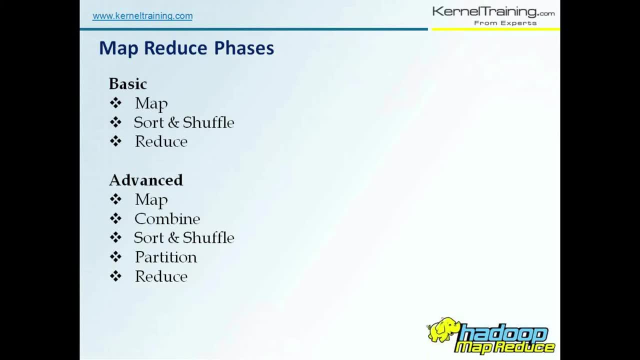 and shuffle mapping. not only that, one and again key value phase, also it makes itself: if it is available key value, it take it. if the data is running text, it automatically generates its own key value, kind of thing like: and again short and shuffle phase when the data is already there. 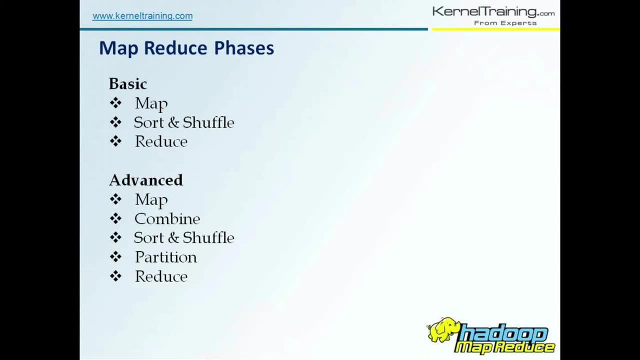 Processing, usually in individual nodes. it has to be sorted the data. finally, it has to be sorted all the data and aggregated and sent to the reducer. So this is what the short and shuffle will do. it groups the data. actually suppose a particular data app will go in one node, all the app in nodes which are there in the different nodes. 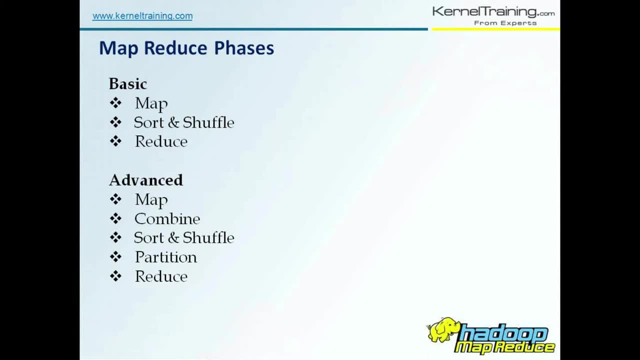 are sorted, and that is what shuffle is shuffled, sorted into, put into the, send it to the reducer. that's what this short and shuffle phase will do And the reduce phase they do. space is still. again. there are: do apple one, apple two, apple, apple, like that, all the five apples will be an apple five. it will find out that way, whatever. 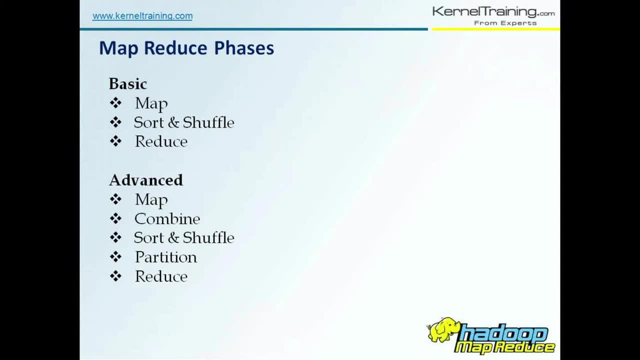 that it has to reduce it. to reduce it again, we use it also. we do short and shuffle. finally, the required output will be generated in both the phases: map phase and reduce phase. user can control, user can give what kind of information they want and they want to sort it out. they. 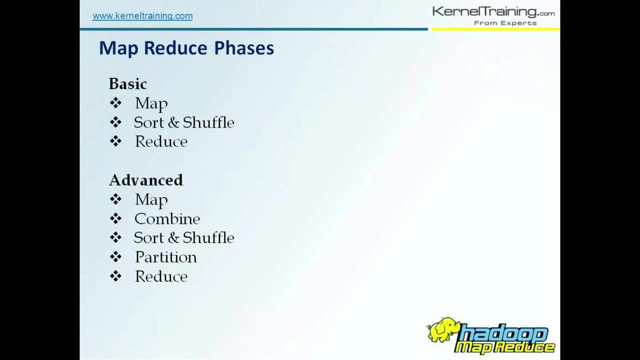 want to count some of the data they can do. they have to extract and do the remove, the do case. they can do that. do whatever way they want, they can do it. that was, and there are two phases also added here in advance of the phases, like in between the map and source of all. 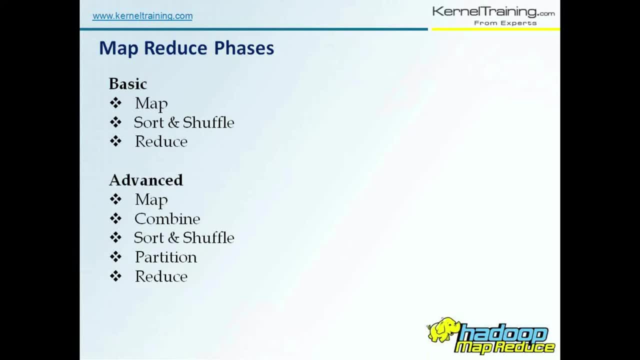 then we combine our phase. what combined we will do is when the- if it's a very huge data, so much shuffle, take what has been standing in bit so you can come by, you can use the, your wall sorting and finally, on the surface, I will be reduced. 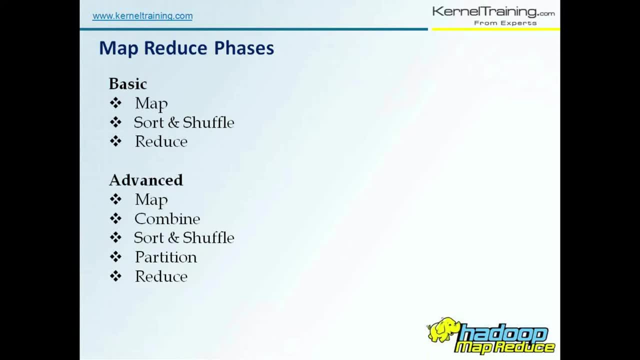 so that it's a network, traffic also reduce because it's a cluster. now it has to keep sending the data from here and there, from this note to that note, this note that only keeps ending in certain couple phase, so that an important coffee can be reducing by combiner, adding one more. that means these are these two. 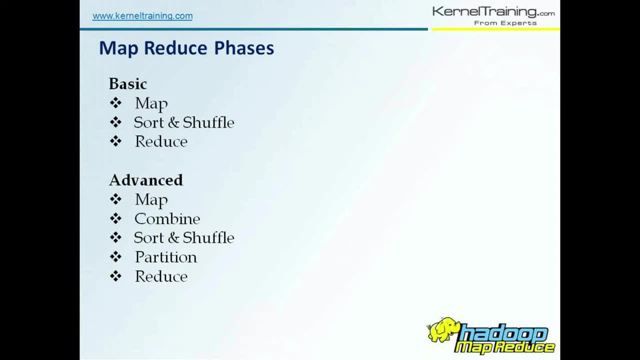 things are, for there is a, there are data available in which about that male and female data it is there, it about the million maybe in from the Mars or any other things like so what you can say that all them, so that there will be two, reduces like a male data will be in the summary. 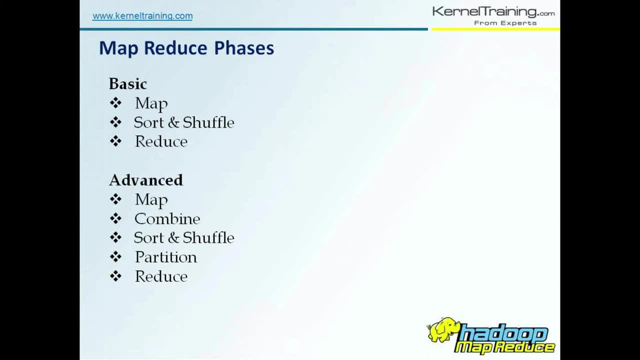 user and the female data in the summary was finally not. this can be easily segregated. this many males have this much a population, this many ways you may have this population or this must literacy anything you want to tell. so again, the button is reduced, like for another user. that way you can separate. 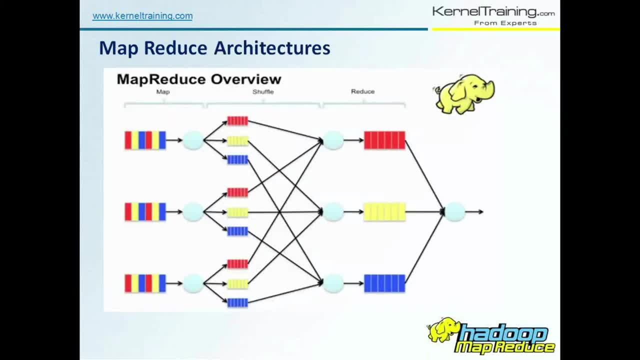 again the. finally, user can separately generate the. you can see it here. these are on the nose here again. this is: the data is fed to here from here, like, and then it is shuffled. see how it is. shuffling is happening. like to the user from data is. 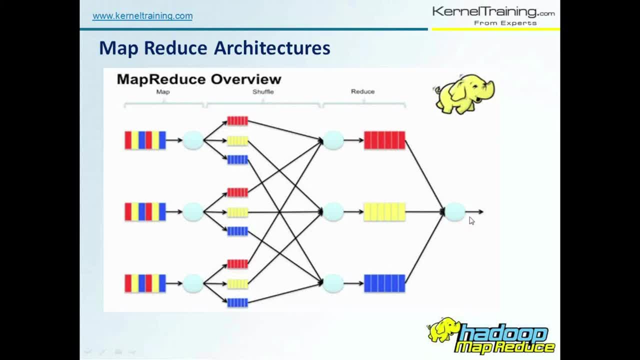 segregated here and finally send group. this is what the concept. but we think that in the detail class we do each phase separately. how detail you need to discuss about see how it leads the data, how we put the data into the data and to the cluster, right the data. all these things you can discuss later. and a small 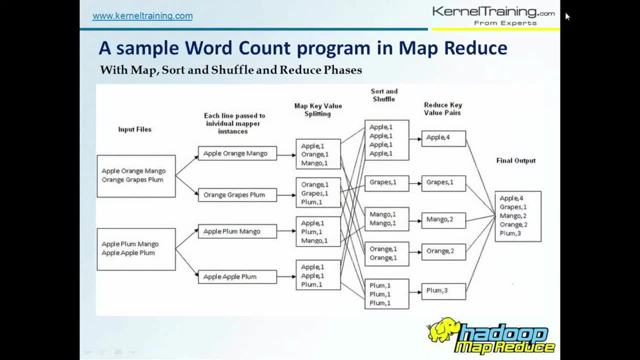 program I have taken. like I said, no, that today is a simple workout problem. if you just give this one how the output is in the attack, you, by seeing this one yourself, we will come to know about our map with user will work. what are the different phases, how the data is passed to the different phases like see there. 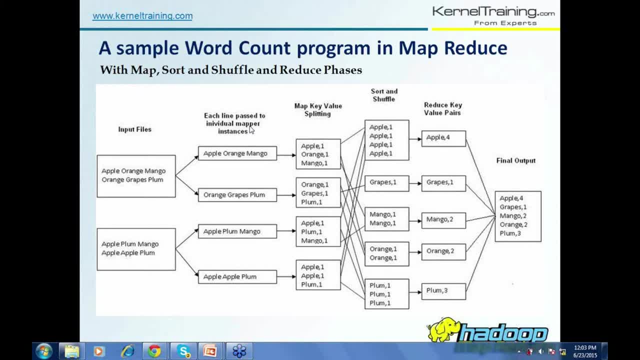 is a pill, or and mango, or and date like that. there is one running test format data. now, within this data, you know to come up, find out what the data is like now, within this data, you know to come up, find out what the data is like. see, there is a. 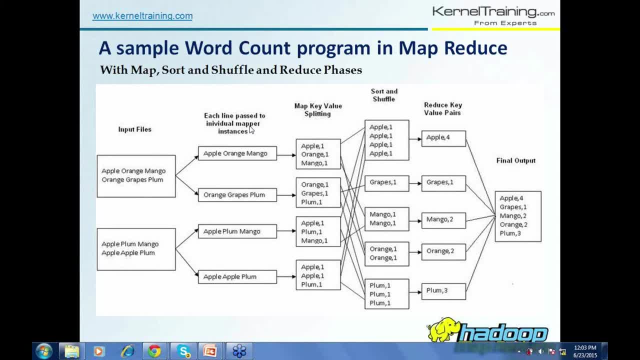 now within this data. you know to come up find out what the data is like. see there is a counter. how many Apple words are available within this file and our orange like mango, like that. so what it is doing now input file is put into the say positive to the individual mapper instances here. see what it will do is. 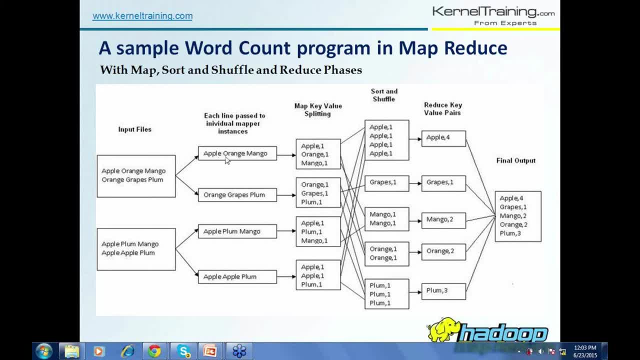 it will generate its own. since it's a running test, it will generate its own kind of key value- is not shown here- actually generate the key value itself and then each line will with key value. value will be this line here: key value. value will be this line here: key value. value will be this line here, key value. 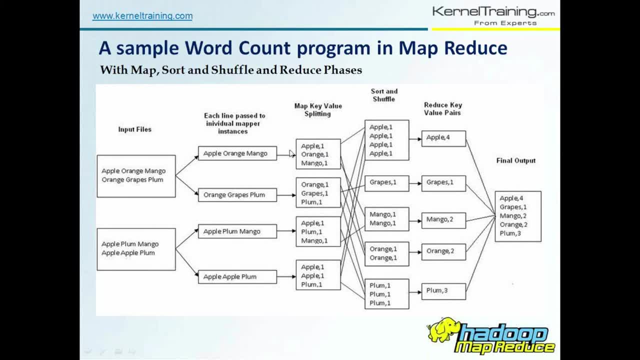 value will be. less like that it will be. and then map key value splitting. then again, after key value, this one, a map will have started splitting that. it take the apple and see how many apples are there here like that, see orange, within this node only, I'm telling, and again, in this node only, what are the things are? 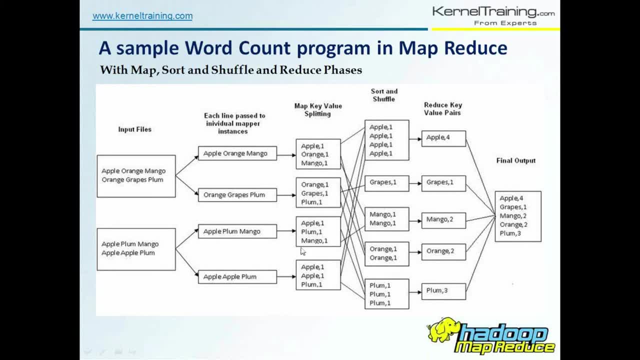 there. so like that, this four nodes individually, the mapper will sort out the data. so again, the mapper will produce, produce the data, not sorting, it will just produce the data. see, hey, map is one here, there may there may be map here also in another same node. it'll write down my apple one, happen to happen. 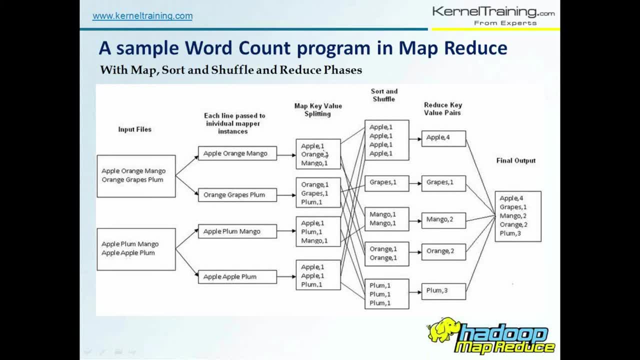 like that happen. one happen like that, you right. and the sort of shuffle face. see all the apples are group would. all the orange are group. all the gray grapes are group. this is what the sort of shuffle phase will do. see all apples from the all the classes is put here like finally reduces job is again it. 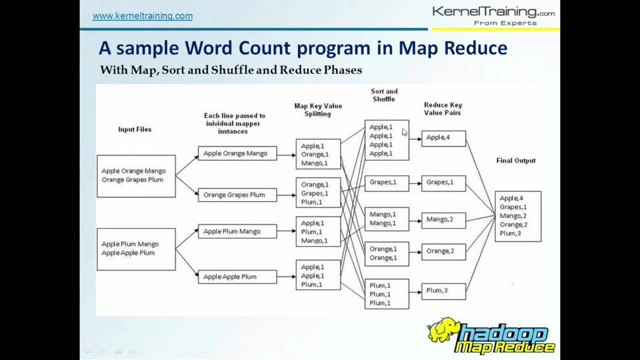 will start out within the appeals. how many are there like count, because this is a work of work of? we have submitted the job, so it will produce that there are four, one plus one plus one plus four. four are the subject. this way in nine. this is one work of job. we are passing similarly. whatever way you want we can. 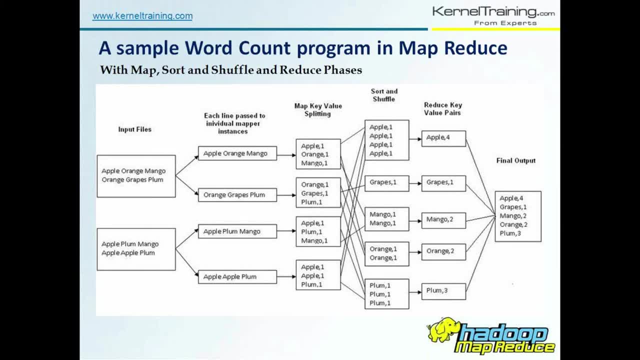 specify the map per face. you can specify the reducer phase also. ending lead. the output is generated. the slot now see. finally, the output is given into the like apples for the grape. one minute, see how it is working. is the same technology working for all kinds of the input format? but thing is like, whatever way you want it, you can. 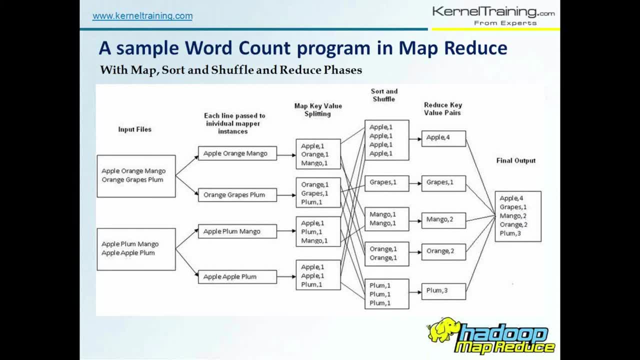 specify in my face and into the face you can write the code and set the, submit the job. how simple it is. you just see, you appreciate, and in between I the last, this one slide has only map, map face out and shuffle and reduce phases. but I discussed about the two other phases now how the data we need passed through that. 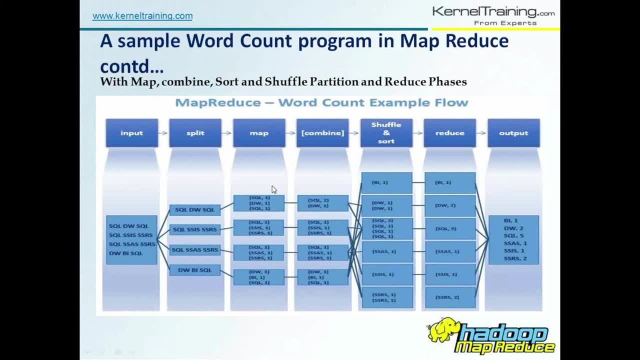 two phases, like in the combine and what one is the combine. other is here there is no partition. actually partition means suppose there is a partition, means here there will be that many reduces. it will be: see now same data. suppose another data is, just take it in the map phase it. 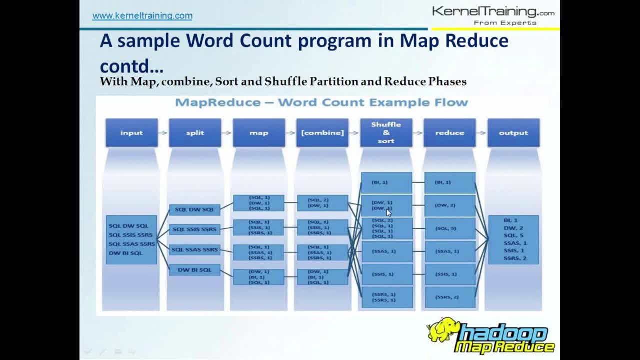 will go like this: and in the combined phase, before that season, the shuffle. what is shuffling is here itself. it is shuffling that one, before going to the shortage of the network. traffic will be very much reduced in this case because some portion of the sorting it will do in the combined phase. and then finally, 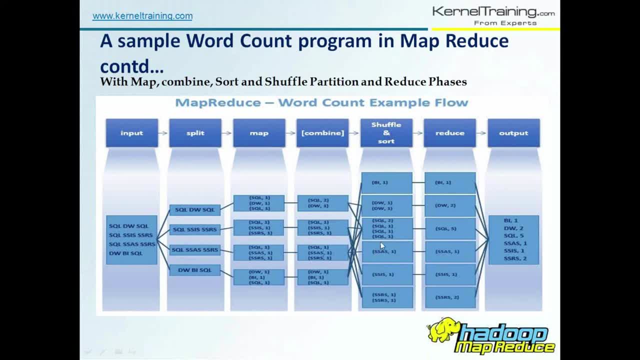 it is, enter the short and shuffle phase, sort of shuffle further, it takes that and it in again further, group it and finally this data is sent to the reducer. suppose in between there will be one partition, that many partitions will be there, that many reducers will be there. 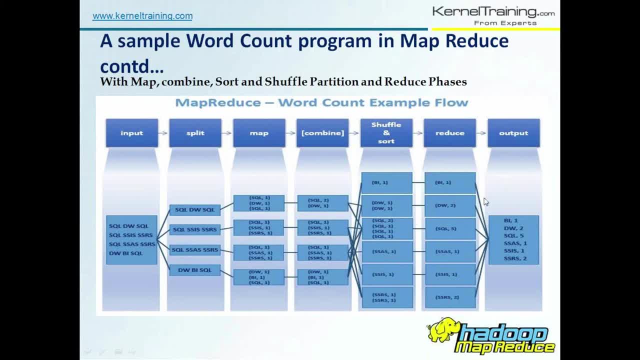 that particular partition data we go to that particular reducer. another partition data will go to the reducer. that way it will be how simple you introduce, because if your data is very huge, network traffic becomes very high and then performance will be degraded. in that case you can decide and then combine yourself, write down your. 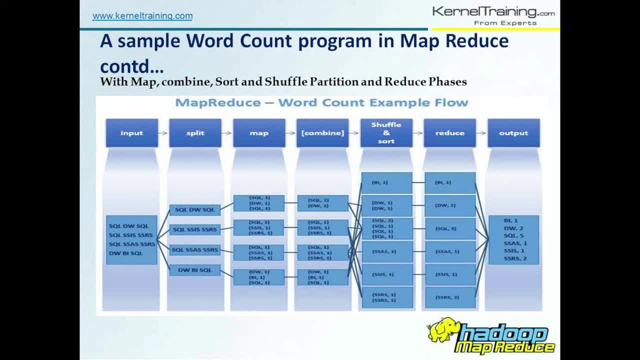 code for that particular data and then combine yourself, write down your code for combining using the Java code and even if you want to partition, you can write the partition as as you wish. if you do not give any combined partition automatically, the framework will take out. take the map phase and sort of. 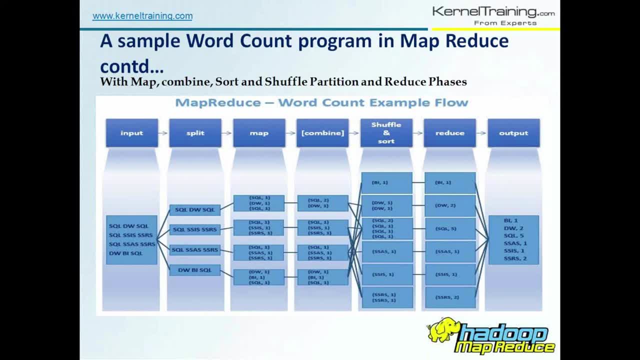 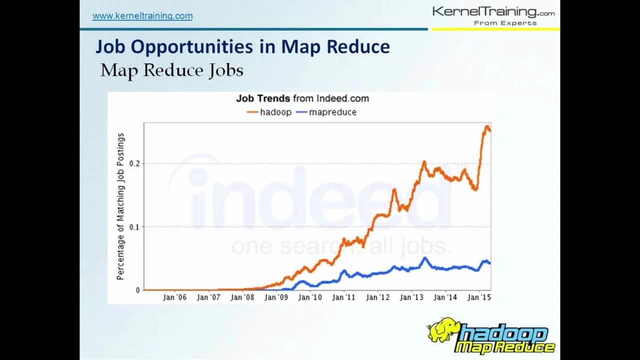 shuffle and reduce phase that way. so flexibilities and finally, what are the Java partitions available in MapReducer? earlier I have shown that Hadoop has a lot of potential antics and it is an emerging technology. everybody, not only big companies, a small company, also looking for the getting the Hadoop projects. 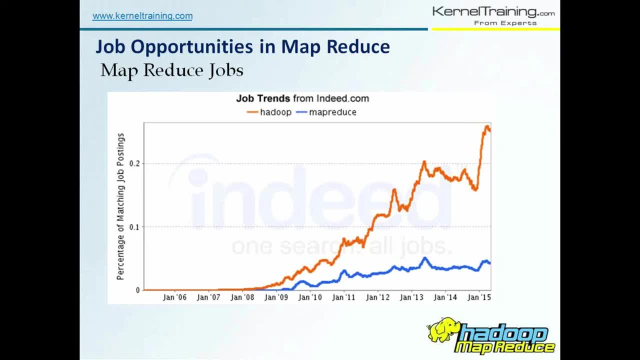 because what they want to do is they want to find out the pulse of the customer: see, when a customer is visiting a shopping complex, what he is purchasing, what are its interests. when the person is visiting a website, what are the website he is seeing. and when he is in social networking, what are the 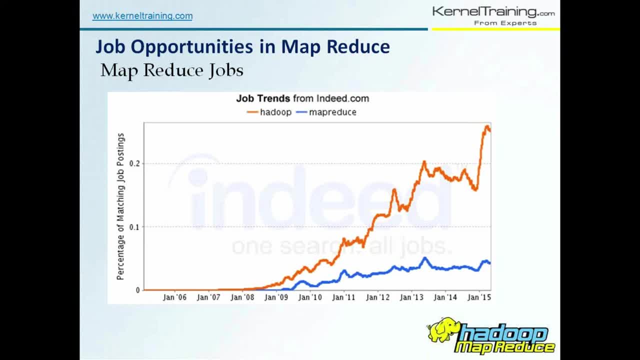 components, what are the products he is liking, all these things, information with them. they want to analyze that. and finally, output to be generated. another interesting thing here: it won't generate simply an output output. if it is generated and dashboards is generated, you need to take the decision like what to 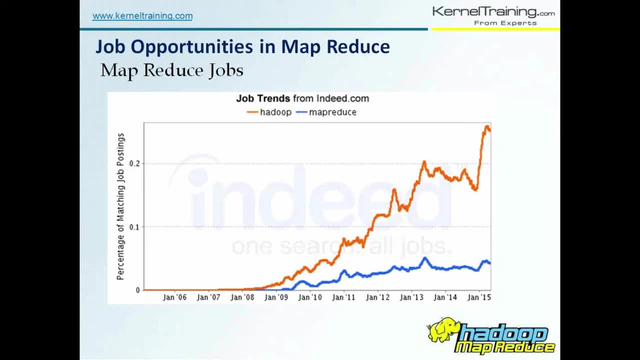 do with this output. so this much area only. it is interested, so I need to market that product. not that it is machine learning language kind of thing. it itself recommends. it itself recommends you go ahead with this one, your business will improve, that kind of thing. see how it is like. so when you are visiting, some websites are thing. 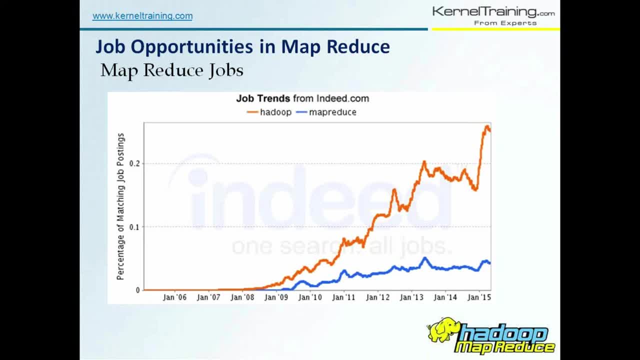 recommended size. they are showing no. that means this is what the Bama produce will do. Hadoop will do. it will see that these are all the recommended size for you. these are the recommended thing kind of thing. so that way, when the data used, data is analyzed and produces results and the business can be very much. 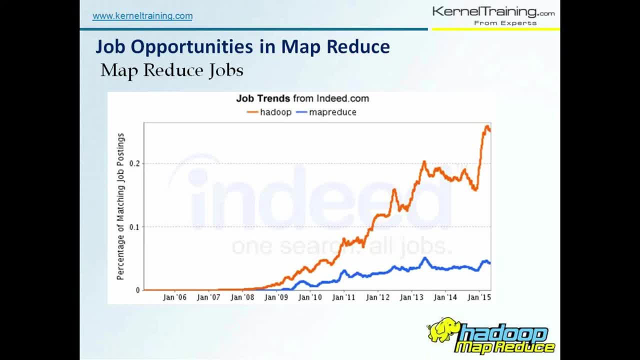 improved. that's what a lot of opportunity seen Hadoop, big data and map reduce and Especially if you are good in MapReduce and Java Java, if you know the Java you can do the MapReduce They appreciate and the passphrase will be given. 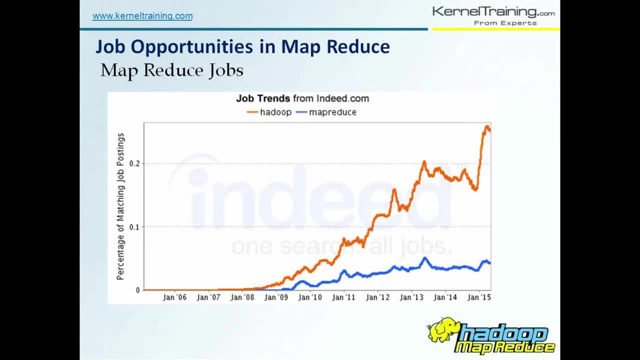 for those who want to go to this job with the MapReduce technology that way. See, you can see the graph also. and how do properties this much Exclusively for MapReduce, this much properties there in the green? you can see that one that way.